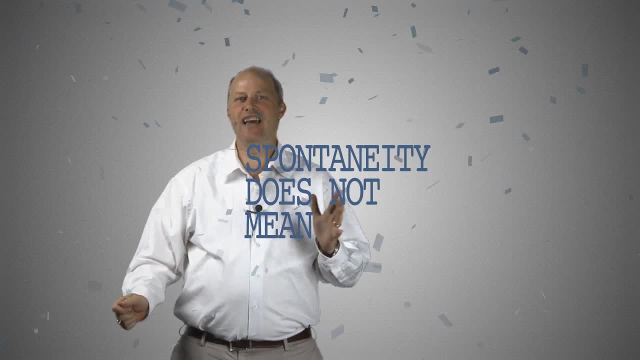 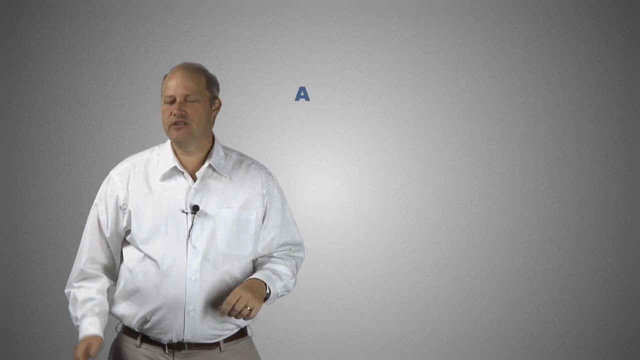 we are prone to throwing confetti or breaking out into dance at any moment, But thermodynamic spontaneity has a very particular meaning. So in thermodynamics we're always thinking about starting at some initial state and going to some final state, If we say that process. 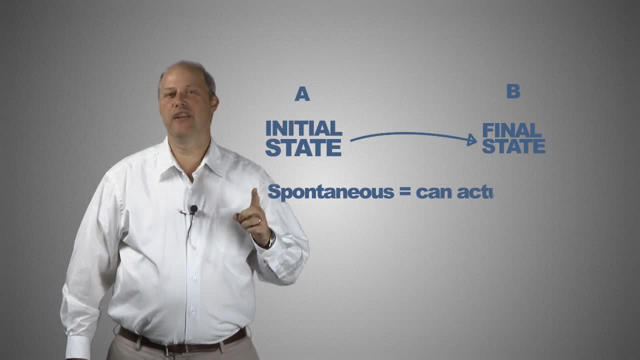 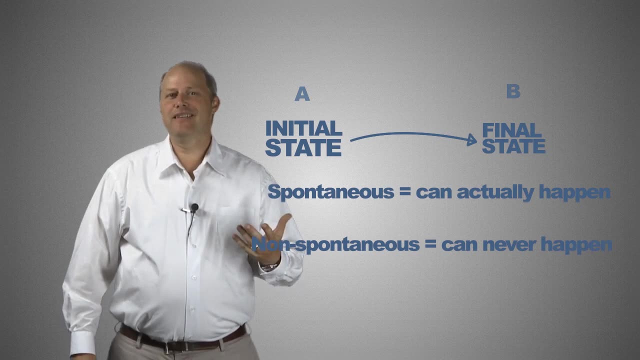 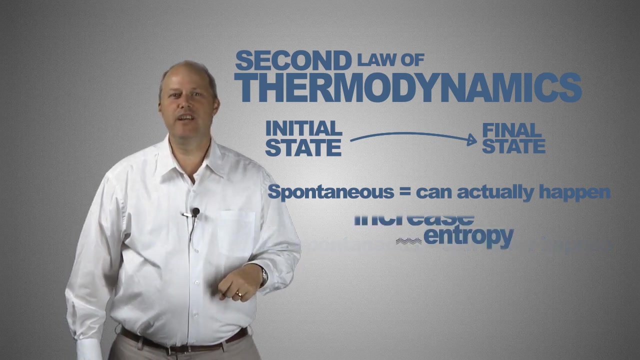 is spontaneous. all it means is that process can actually happen. Things that are non-spontaneous are things that can never happen, And the reason this is is the second law of thermodynamics. So spontaneous processes, processes that happen, are things which increase the entropy of the 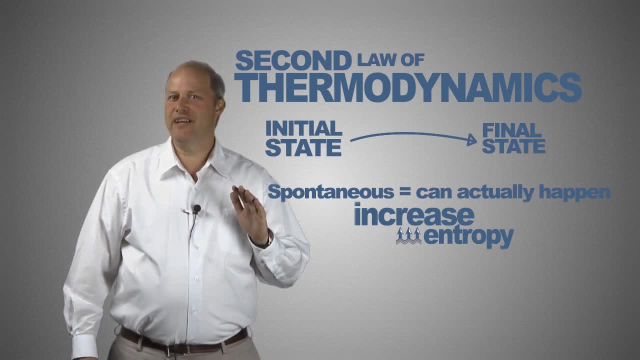 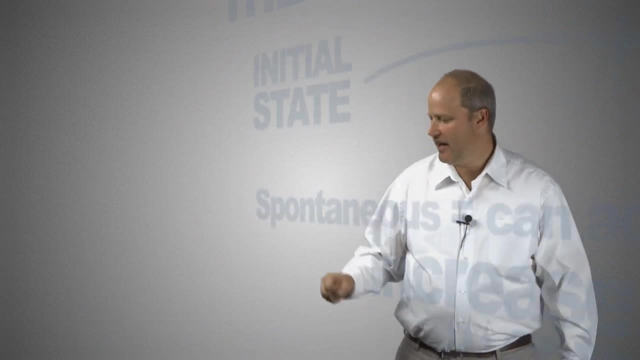 universe. Now it sounds very complicated, but it's actually something that you have a lot of intuition for when you're looking at things that happen in the everyday world. So let's imagine I had a brick. I had a brick in my hand and I was to let go of the brick. No one would be surprised. 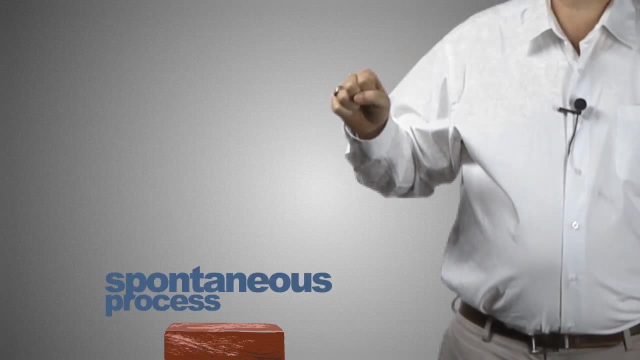 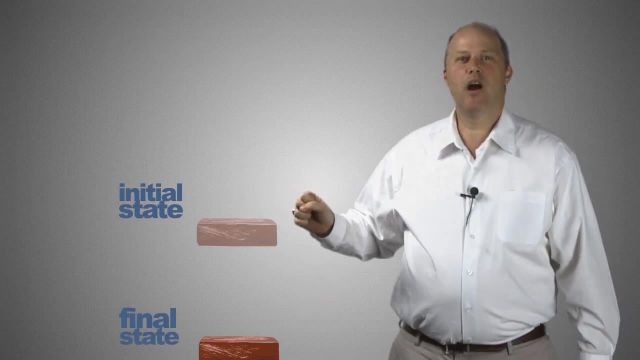 at all that the brick falls to the floor, because that's a spontaneous process. So the initial state is the brick in my hand, the final state is the brick on the floor, and that happens without any problems. But I can stand with my hand over the brick for as long. 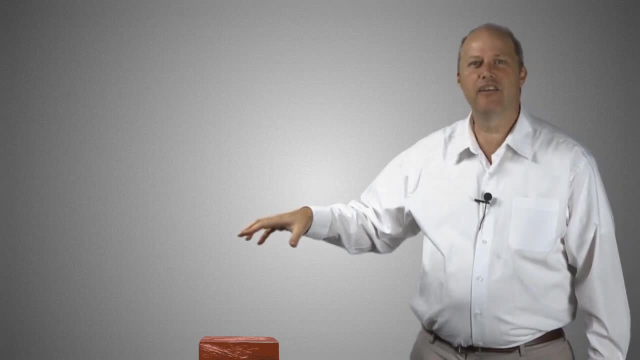 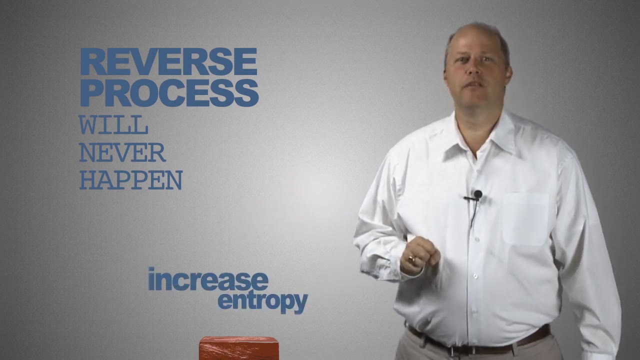 as I want, hoping that it will fly back up into my hand. But the reverse process will never happen, And that's because dropping the brick increases the entropy of the universe. The energy that was stored in the potential energy of the brick is converted into kinetic. 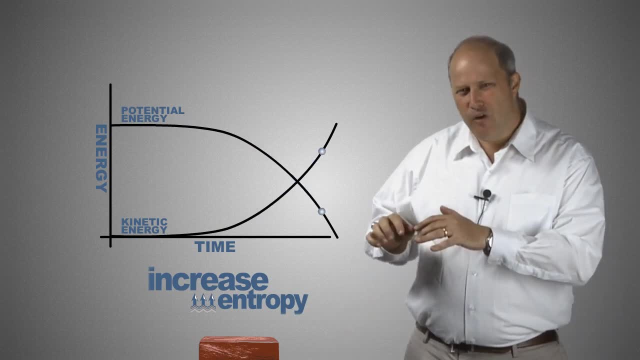 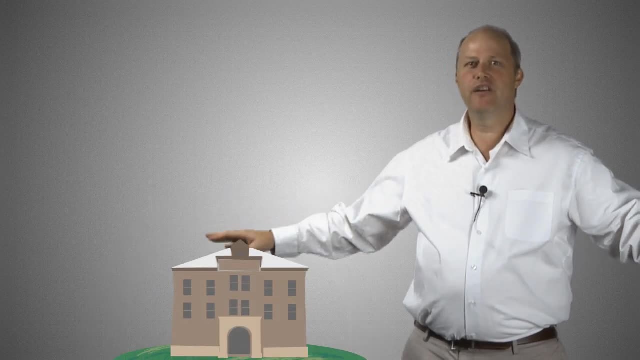 energy. as the brick falls, And then, as the brick hits the ground, that energy is dispersed in vibrations in the floor and then vibrations out into the building, and then vibrations into the ground and then out to the edges of the universe. I can wait as long as I want. 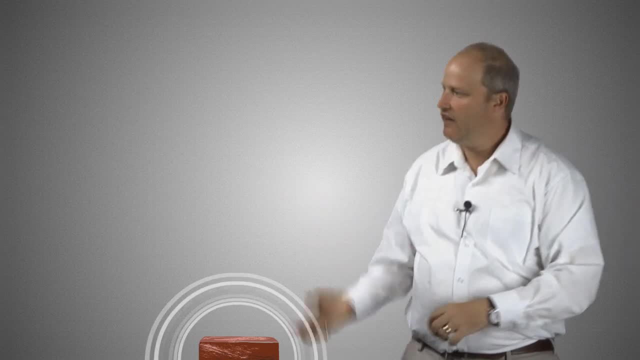 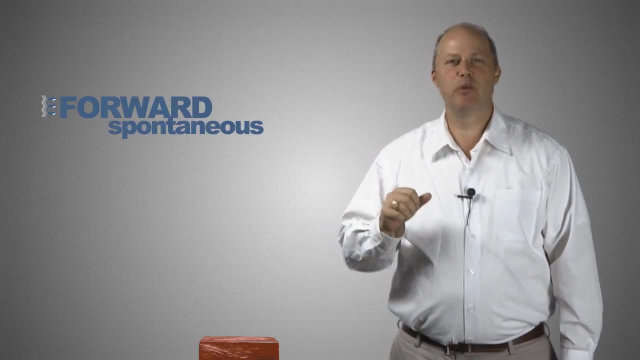 for that energy to come back and concentrate under the brick and fly up into my hand, but it will never happen. I can wait as long as I want for that energy to come back and concentrate under the brick and fly up into my hand, And that's because the forward reaction is spontaneous, but the 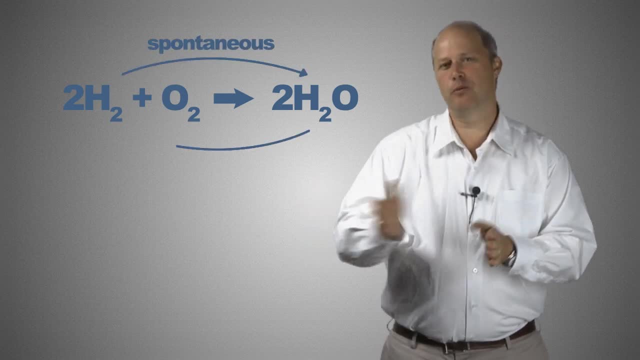 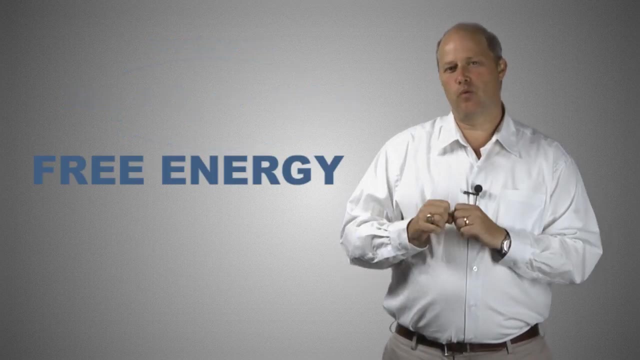 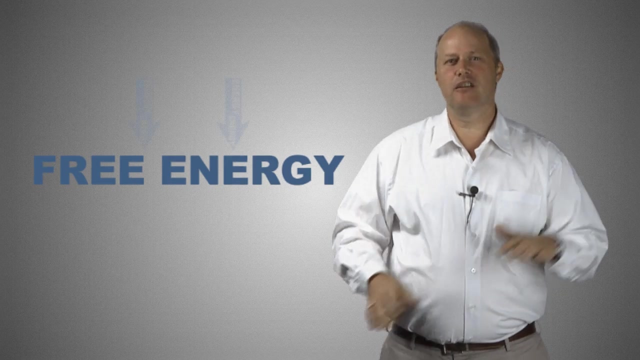 reverse is not. Now it's much more difficult to look at a chemical reaction and just say, a-ha, the forward is spontaneous but the reverse is not. But thankfully we have a way to calculate that. So we've invented this idea of free energy which wraps up all of the entropy changes.